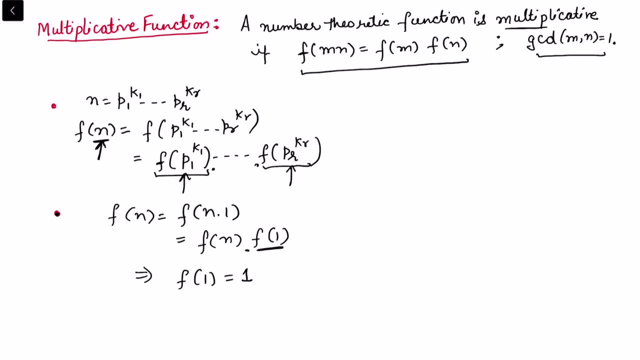 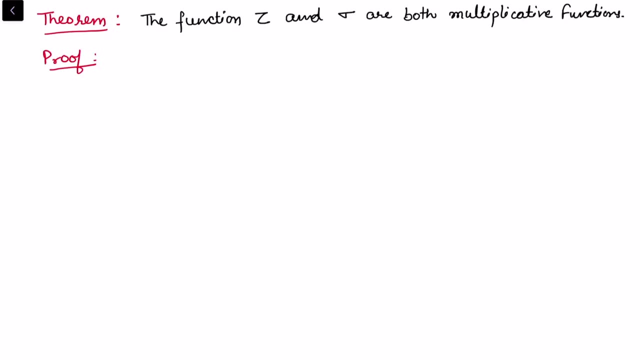 If it is zero. zero into this function will make the left hand side also zero, which is not the case. Considering that fn is a non zero function will say that f of one is identically equal to one and f of one is not identically zero if it is given that f of n is not equal to zero. Next we prove the function tau and. 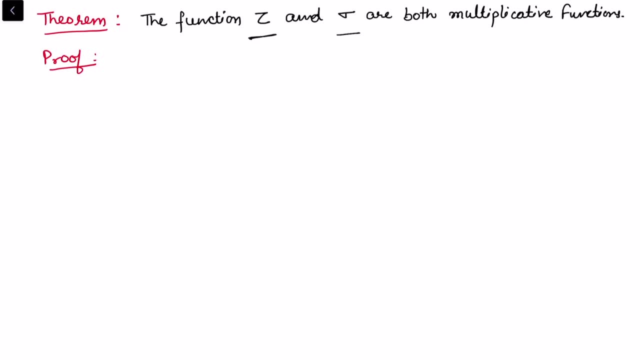 sigma both are multiplicative function. Tau n is this number of divisors, sigma n is the sum of divisor. And let's now what we want to show. we want to show for the multiplicative function: tau of m of n is equal to tau m into tau n, whenever the gcd of m and n is equal to one. 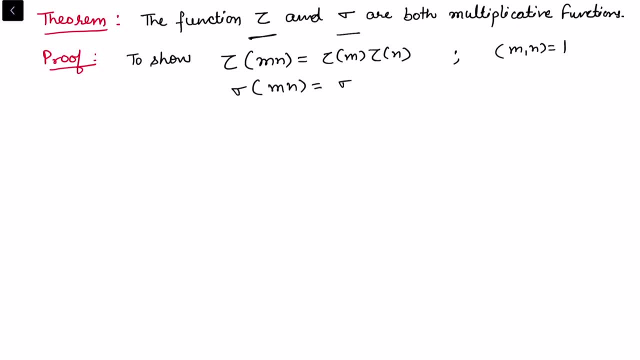 Similarly I want to show sigma of m of n is equal to sigma m into sigma n whenever the gcd of m and n is equal to one. Now let's prove the first case. For the first case I'm also going to consider first the prime factorization of m and n. 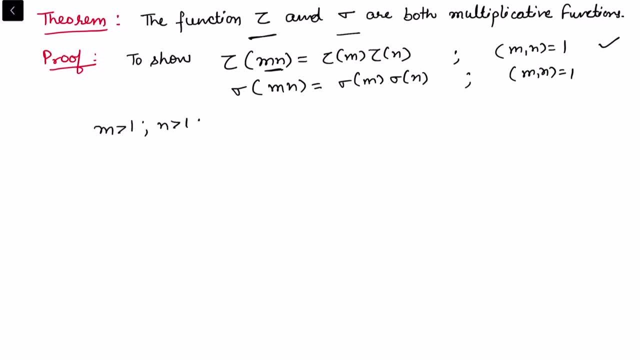 So let's take: m is greater than one and n is greater than one. Let's take non trivial cases, Because if any one of them is equal to one, the gcd is automatically going to be one. So, considering the non trivial cases, m is greater than one and n is greater than one. 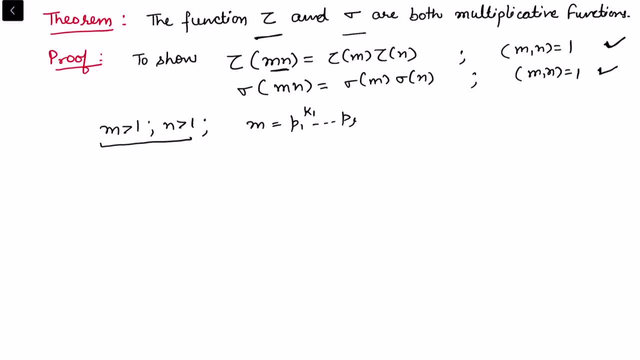 And I'm also going to take the prime factorization of m. let's say this is the prime factorization of m and let's say n has this as the prime factorization. We must need to take distinct prime because we have already said that the gcd of m and n is equal to one. 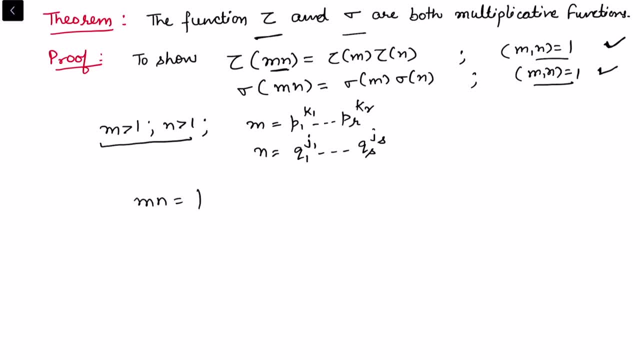 So this means m and whenever I take the product of this, so all primes will come because they are distinct prime. So let's write down this: So this is the all prime here: j1 up till qs, js. Now let's apply tau of m, n, and we have already done, by the definition of the tau n formula, that I've done in the last video. 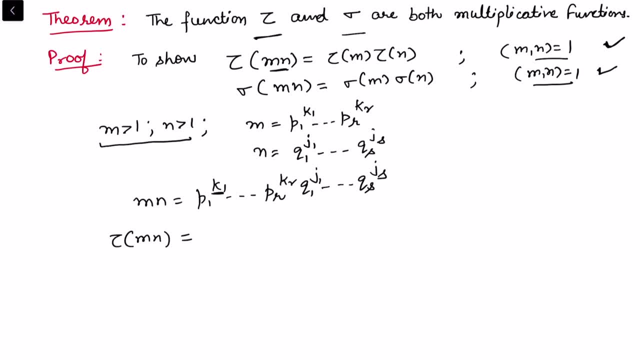 This is: whatever be the prime coming, Look at the power of the prime and then just add one more to that, So this would become the formula for tau n. So just applying the formula for the tau n function, and this will continue: j1 plus one. for the remaining primes also, js plus one. 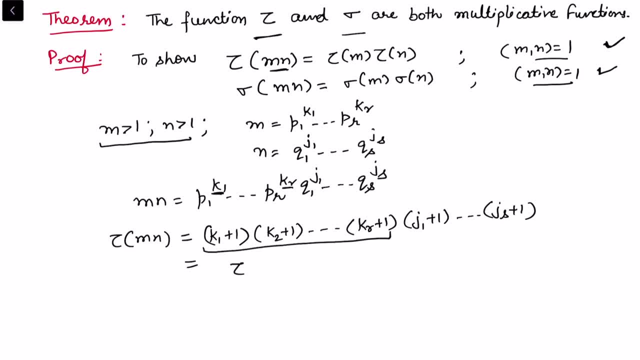 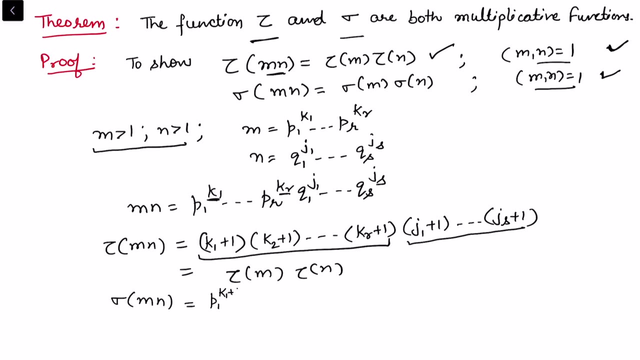 Now this is same as this expression is same as tau of m and this expression is same as tau of n. So this result hold, saying that tau is a multiplicative function. Similarly, let's apply the formula for sigma m n. Sigma m n have a formula: p1 to the power, k1 plus one, minus one upon p1 minus one, into p2, k2 plus one minus one upon p2 minus one, and so on. 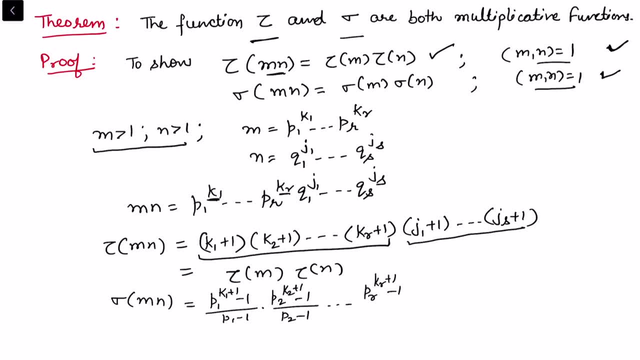 pr to the power kr plus one minus one upon k2 plus one. So this is the formula j1 minus one upon pr minus one, and continue this for this expression also j1 minus one upon q1 minus one, and so on qs, js plus one minus one upon qs minus one. 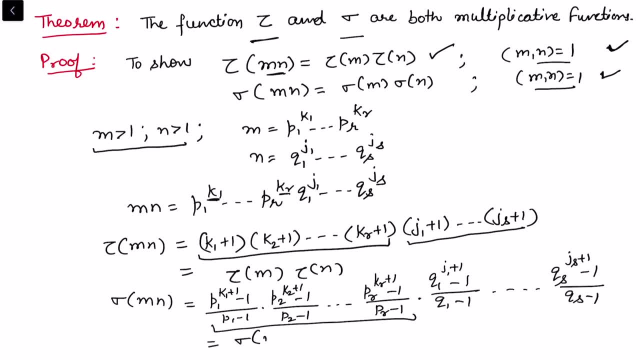 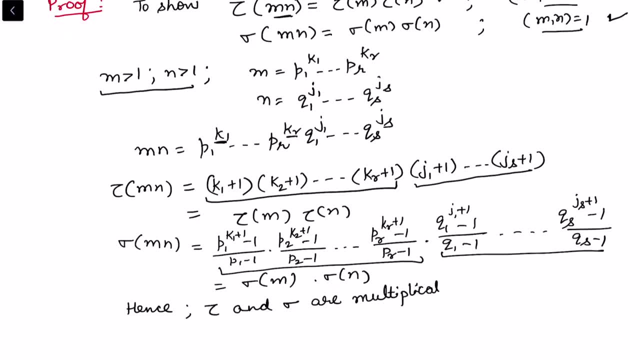 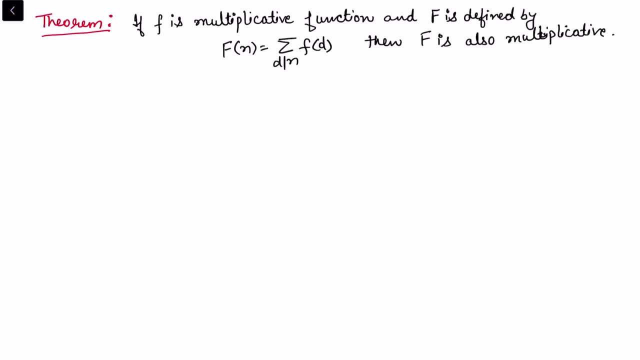 Now this is same as sigma m. The other quantity is same as sigma, So hence we can say tau and sigma: both are multiplicative functions. Now we prove our third result, as mentioned in the objective of this video. If small f is a multiplicative function and capital F is defined by this expression, 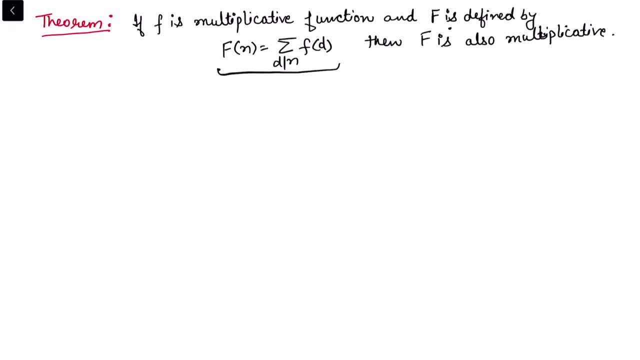 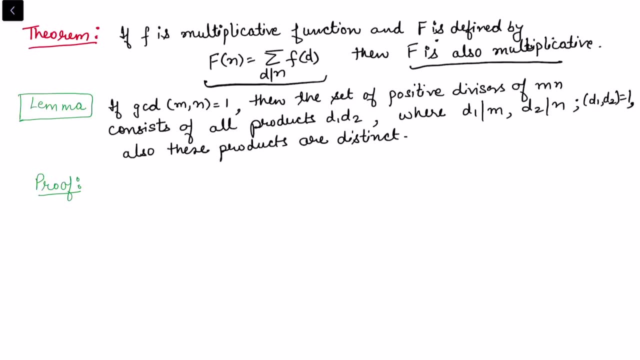 That capital F is summation of fd. d divides n, Then capital F is also a multiplicative function. Now to prove this theorem I am going to use a lemma. So let me to state the lemma. First lemma: state: if gcd of m and n is equal to one. 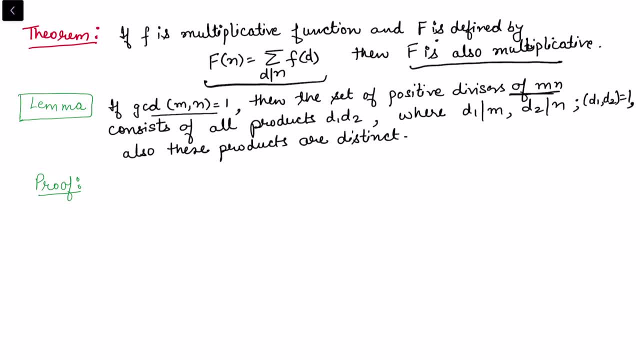 Then the set of positive divisors of m- n consist of all products of d1- d2, where d1 divides m and d2 divides n and d1- d2, gcd is equal to one, And all these products are distinct. So now let's start the proof. 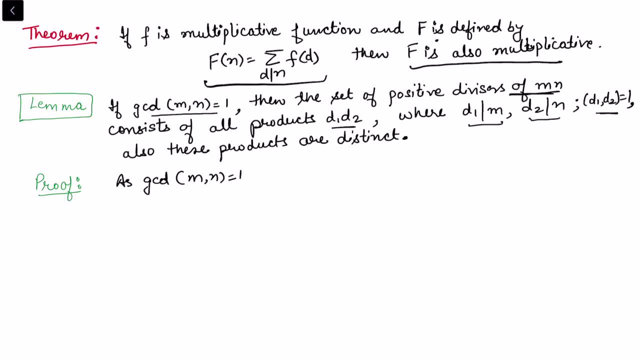 As gcd of m and n is equal to one And we want to consider a divisor d of m- n, Let's consider first the prime factorization of m. Suppose m has this prime factorization, And let's take n also has some prime factorization. j1 up till qs, js. 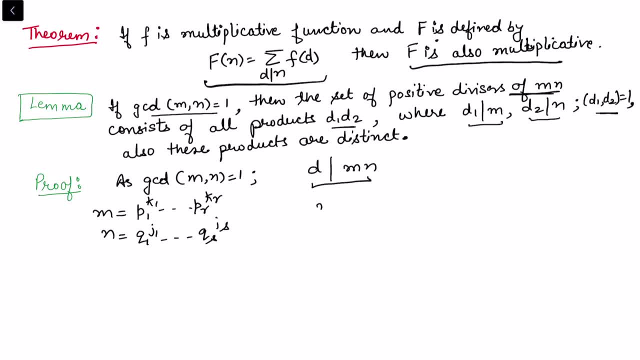 Now, as we have considered that d divides m? n, So this means m? n can be written in the form of the prime factorization, And we have already done. Whenever d divides this product, m? n, So d will also take the same prime representation. 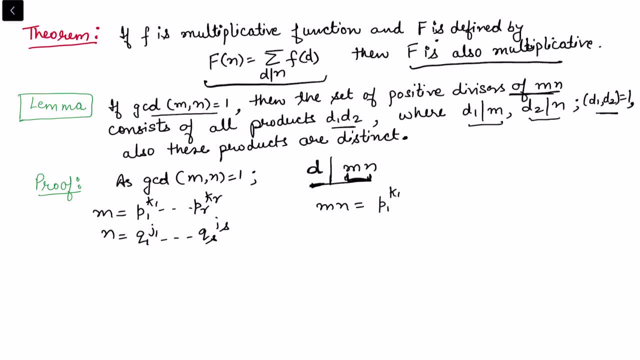 So m n is p1 to the power k1 up till pr to the power kr, q1 to the power j1 up till qs to the power js. This is just multiplying these two, And d will also take the same prime factorization form. 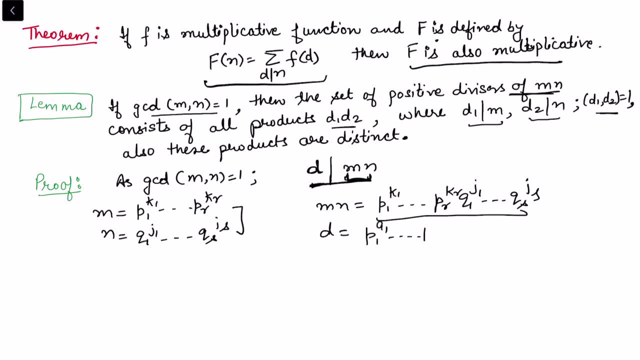 So this means d will take p1 to the power a1, up till pr to the power ar, q1 to the power b1.. qs to the power bs Where there is an bound on ai's. So each of ai is less than or equal to ki. 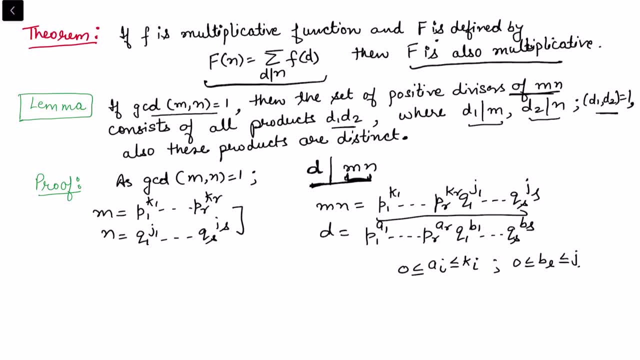 And each of bl's is less than or equal to jl, Here i varying from 1 to r And here l varying from 1 to s. Now, considering that d is in this form, But we can see that pi's and qi's are distinct prime. 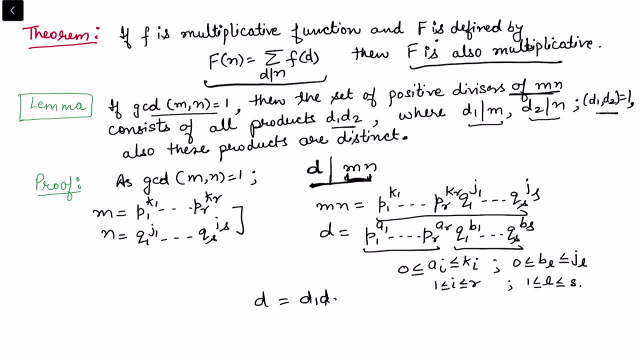 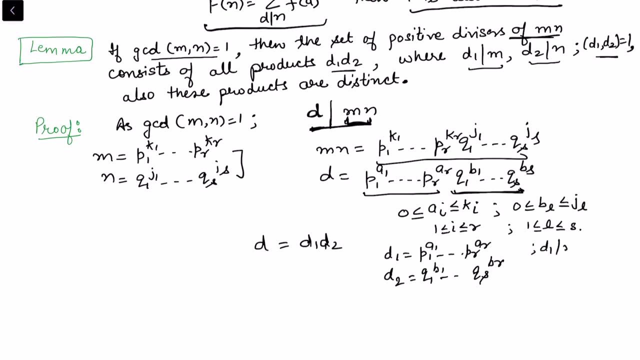 So obviously I can write d also as d1, d2.. And we can see that d1 has a prime factorization: p1, a1 up till pr ar, d2 is q1, b1 up till qs, bs. And from here we can see that d1 divides m and d2 divides n. 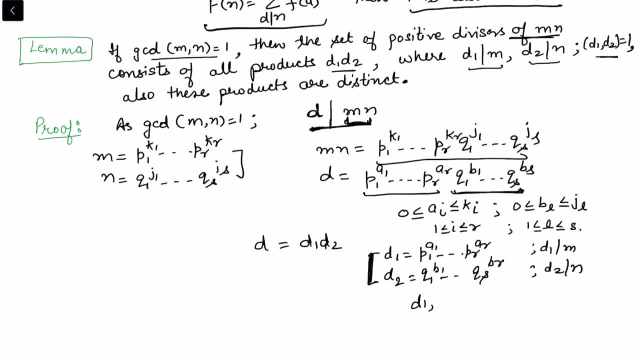 And by looking at the prime factorization one can say that d1 and d2 gcd is equal to 1.. So that proves our result that whenever we have m and n, which is equal to 1. The gcd is equal to 1.. 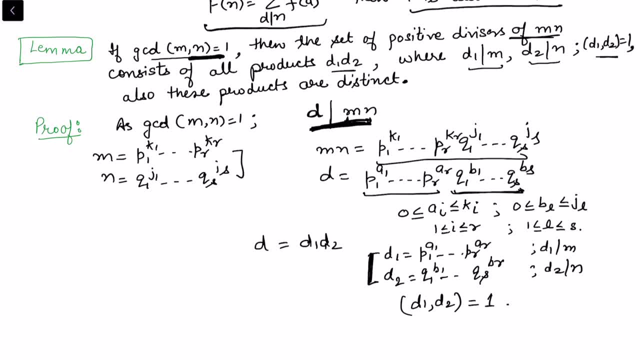 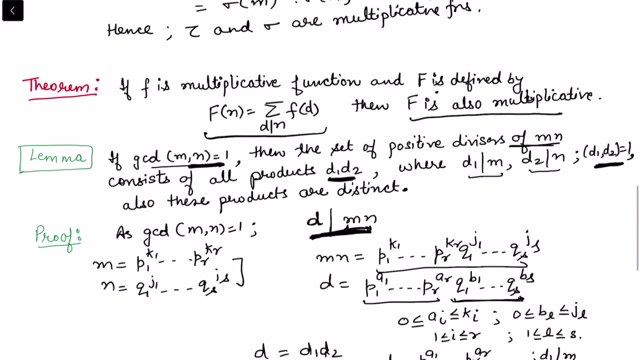 Then any divisor of mn will also have a prime factorization in the form d1, d2, whose gcd is further equal to 1.. So now I am going to use this lemma to prove this theorem. Now let's prove this theorem Now. what we want to prove is we want to prove that f of mn- this is multiplicative. 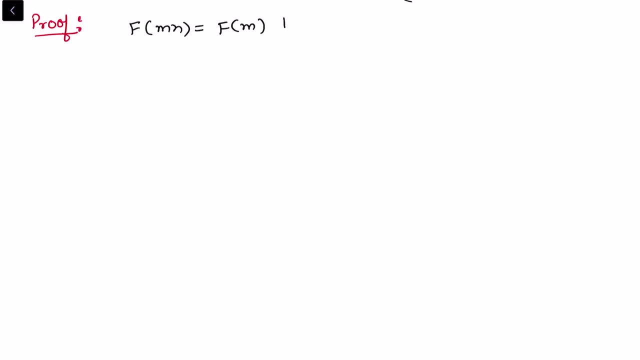 So this means f of mn should be equal to f of m into f of n. Whenever gcd of m and n, this is equal to 1.. This is what we wish to prove, And let's write down now the definition of fm. This is given as what is given to us is fn. 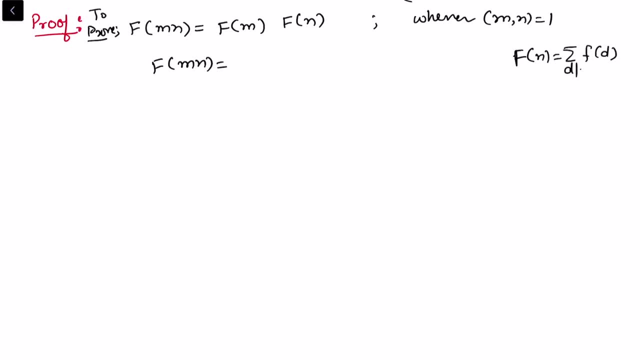 This is written as summation f of d. d divides n. Now, by just looking at this expression, let's convert this inside. we have mn now, So this is summation d divides mn. f of d, And we have seen that whenever d is a divisor of mn and whenever mn is equal to 1.. 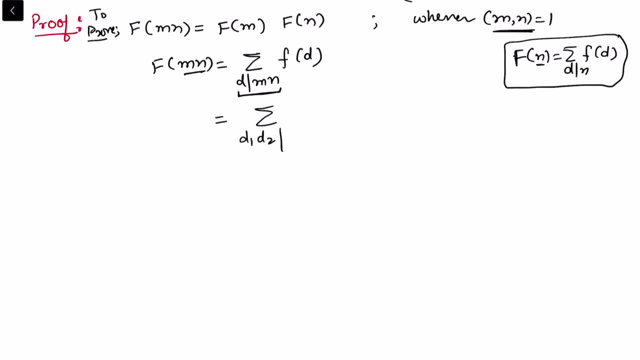 So this can be written as d1, also have a expression: d1- d2.. mn f of d1- d2.. And we have seen that the gcd of d1- d2 is 1.. So there is a prime, There is a divisor, d that divides m. 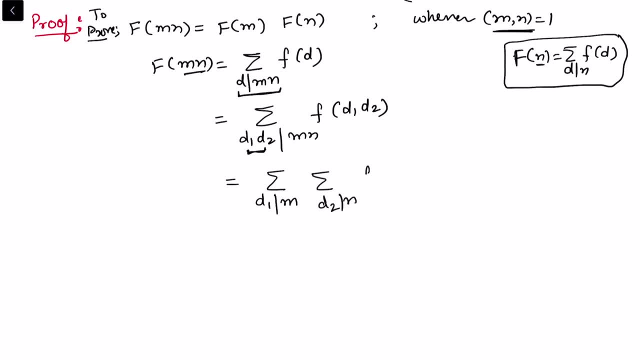 And there is a divisor, d2 that divides n. f is already multiplicative. Small f is given to be multiplicative. We want to prove capital F to be multiplicative, Since small f is multiplicative. so I can write this as f of d1 into f of d2.. 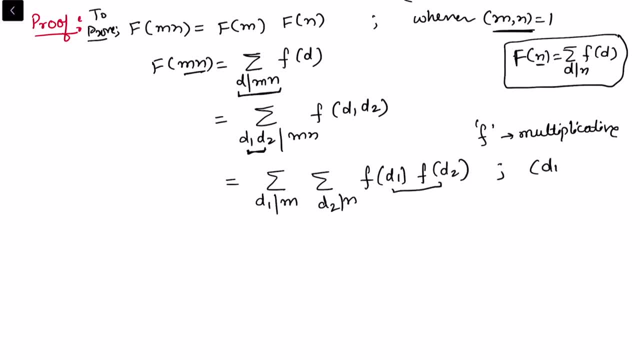 And this expression can be written only when that d1- d2- gcd is 1.. Because we are trying to split this term d1- d2.. And we have just seen from the previous last lemma that d1- d2- gcd is 1.. 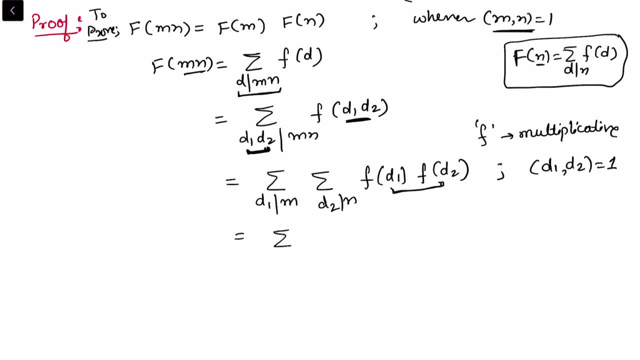 So I can split this expression. This is same as summation d1 into m. Now this sum runs over d2.. So you can take f of d1 here and this as summation d2 runs over n f of d2.. This expression now again matches with this one. 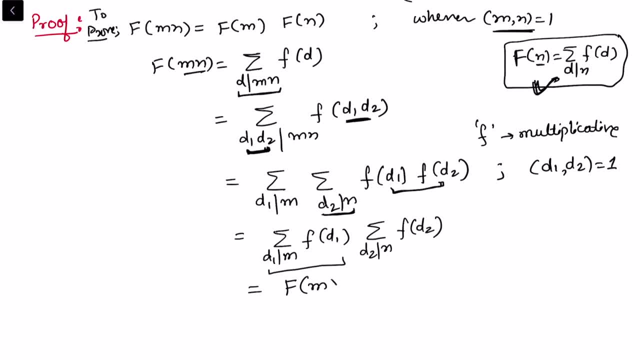 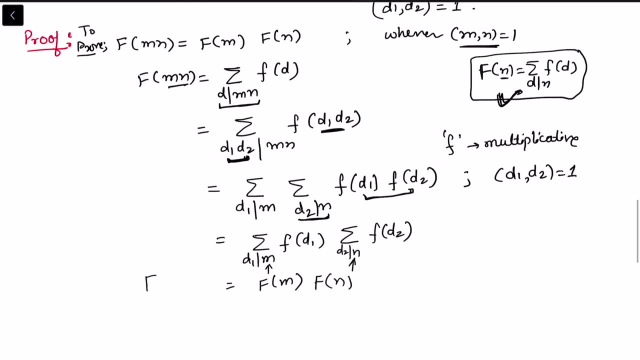 And in this case it is becoming capital F of m, Because here we have now m And the second expression contains n. So this expression will become f of n, And on the left hand side we had f of mn. So this ensures that f is a multiplicative function. 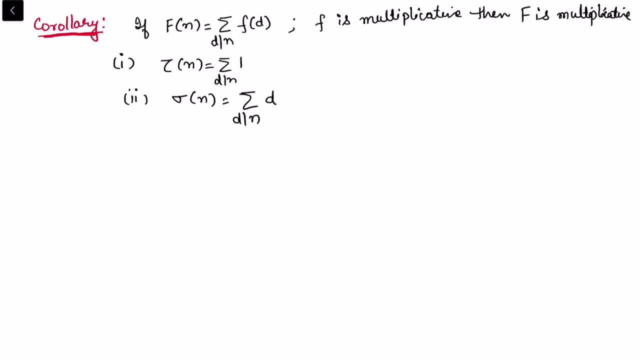 So now, based on the previous result, we can have this corollary- I am considering f and small f, the same expression related by this one- And if f is multiplicative, then capital F is also multiplicative. We just have proved. Keeping this in mind, we can say that tau n is written as summation: d divides n: 1.. 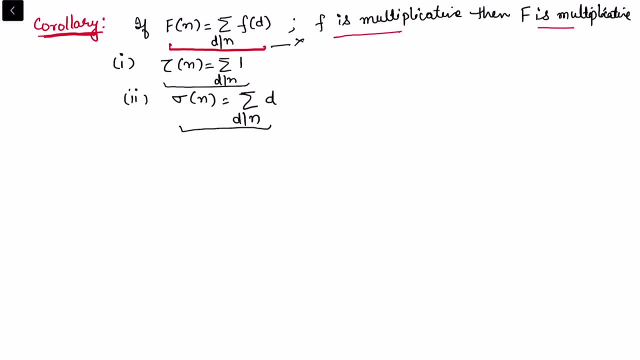 And sigma n is written in this form, Which is the given star expression, And hence tau and sigma are multiplicative function. So now let's take this as the another proof that we have already done. So if I just prove, this results as a corollary of our main result. 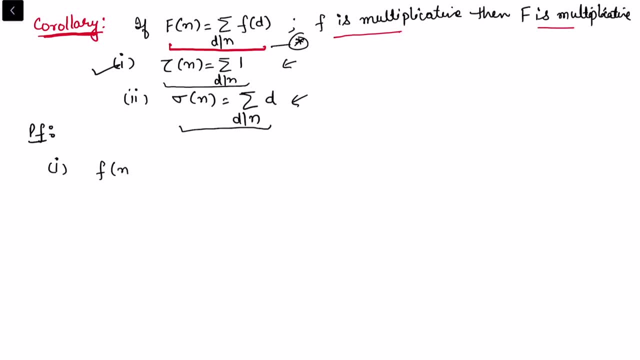 So to prove, let's consider in the first case small fn as 1.. And take capital F of n as tau n. In this case, when I replace this from the star expression, Capital Fn is tau n. Summation d divides n. 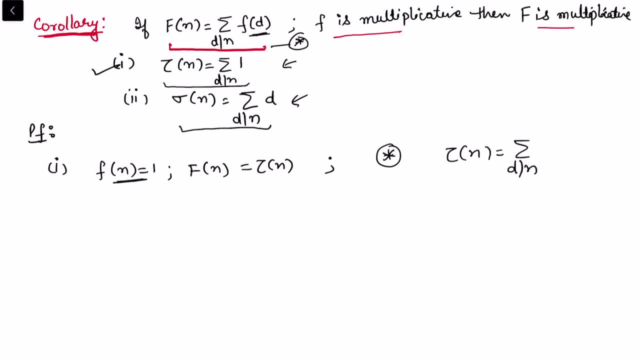 And f of d, Because f of n is equal to 1, so it's a constant function. So even for d also it is 1.. So here this value is 1.. So that is the expression for this case, And we can see that f of n is equal to 1.. 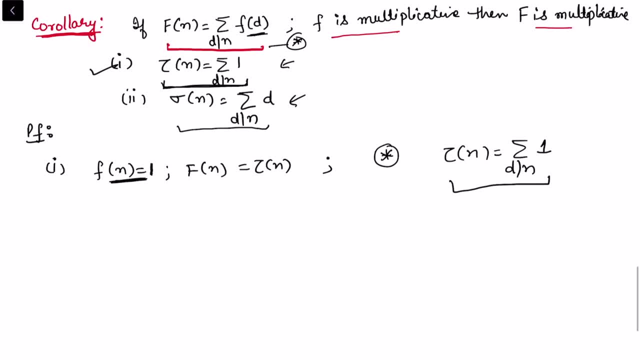 This is definitely a multiplicative function. In this case, automatically. if 1 is multiplicative, tau n is multiplicative. So from this is an alternate proof to what we have already proved, that tau n is a multiplicative function. Similarly, second case. In second case, fn.